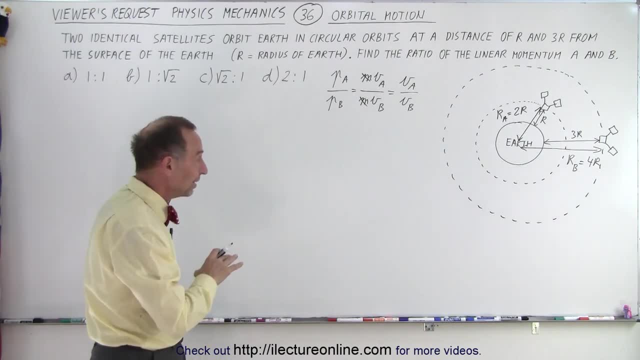 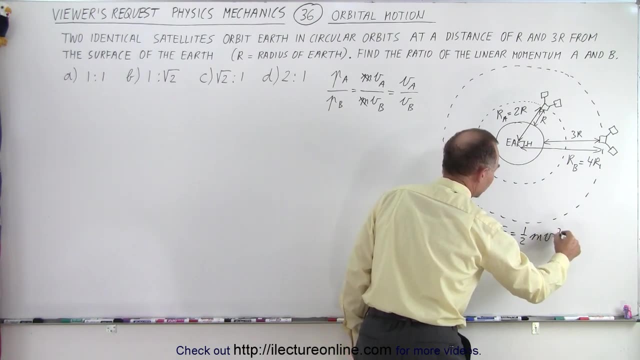 then we also realize that there's a relationship between the velocity and the kinetic energy. we know that the kinetic energy of any object is equal to one half m v squared, which means that the velocity of a and b can be found by finding the kinetic energy of the satellites. 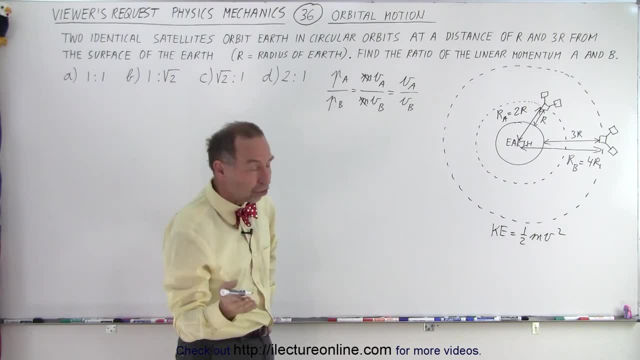 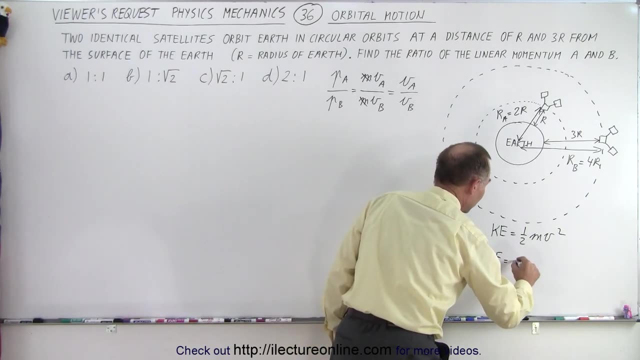 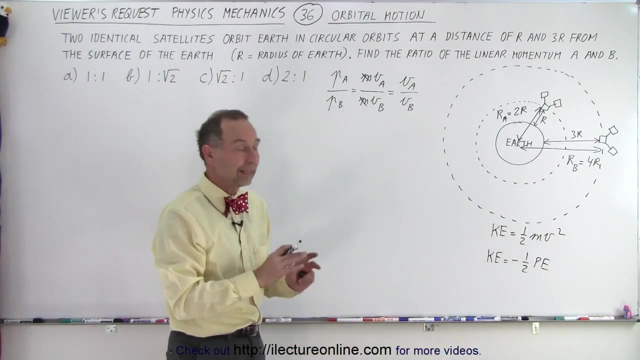 and then we realize there's a relationship between the kinetic energy and the velocity energy and the potential energy of a satellite. we know that the kinetic energy of a satellite is equal to negative one-half times the potential energy of a satellite. so all we have to do is find the potential energy. then we can convert it to kinetic energy. then we can find the velocity and then we can find the ratio. so that's the plan of attack. so the next what we need to do is, of course, find the potential energy of a satellite, And the potential energy of a satellite in orbit is equal to minus the gravitational constant times the mass of the satellite times the mass of the Earth divided by the radius. 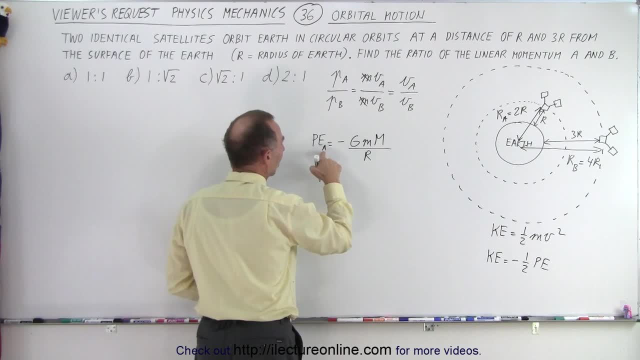 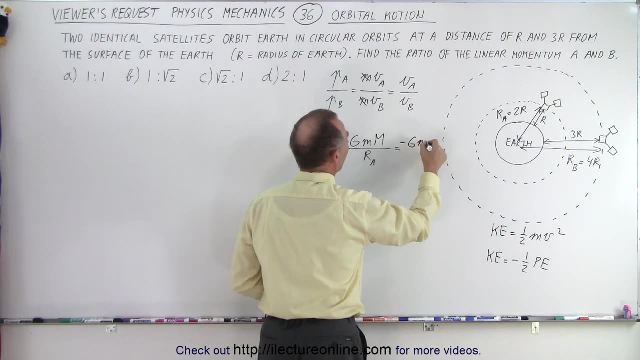 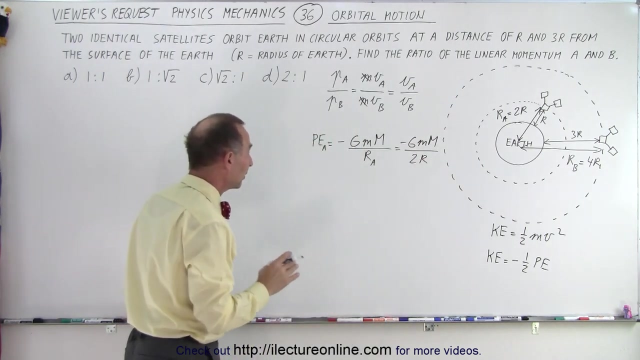 And since we're talking about the potential energy of A, we use the radius of A. So that would be the radius of A, which is equal to minus GM, big M, over the radius of A, which is 2R. Now we can do the same for the potential energy of B. 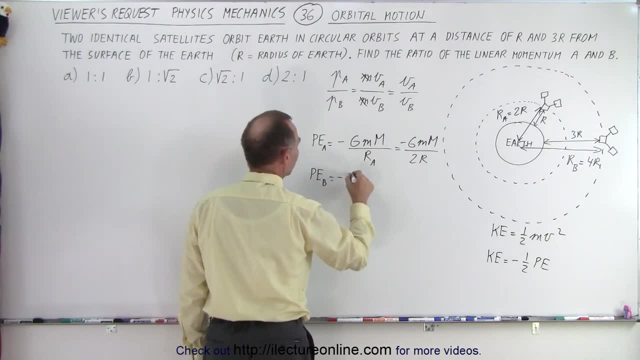 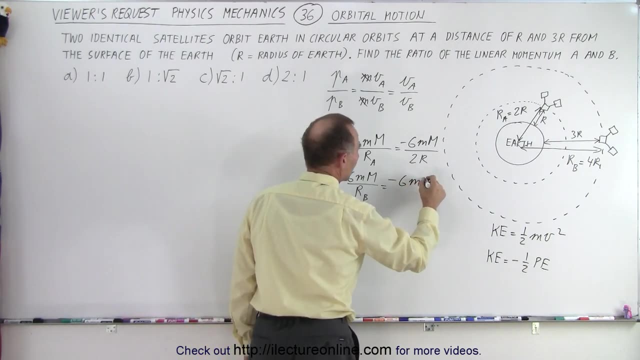 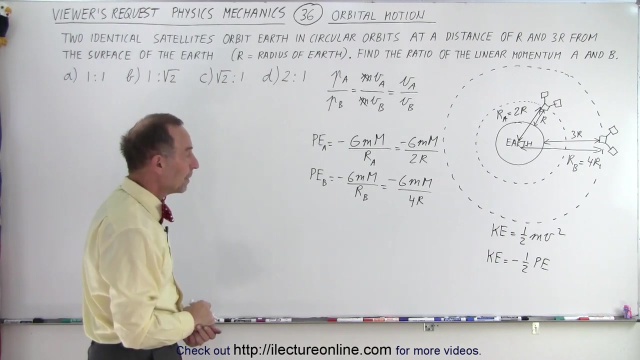 So the potential energy of B is equal to minus GM big M over the radius of B. In this case the radius of B can be found to be equal to 4R. So now we have the potential energy of both satellites. Now we can find the kinetic energy by taking negative one half times the potential energy. 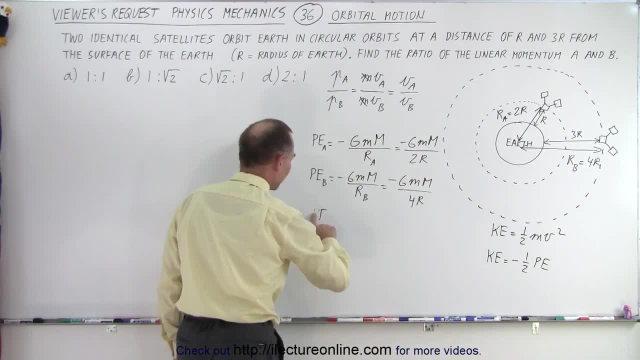 which means that the potential energy- not the potential energy but the kinetic energy- for A is negative one half, so the negative drops out and it's half of that. so it would be GM, big M over 4R, And the kinetic energy for satellite B is half the negative half of this. 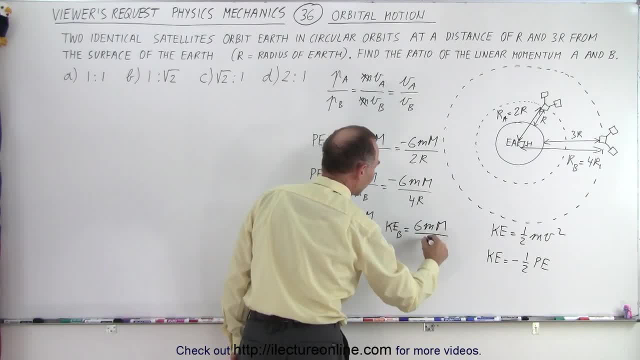 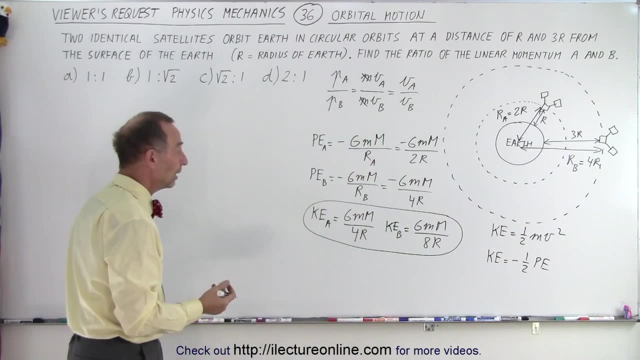 so that would be equal to positive GM, big M over 8R. So now we have the kinetic energy of the two satellites. Now what we could do is we could find the ratio Of the kinetic energies of A to B. So the ratio of kinetic energy of A to the kinetic energy of B is equal to. 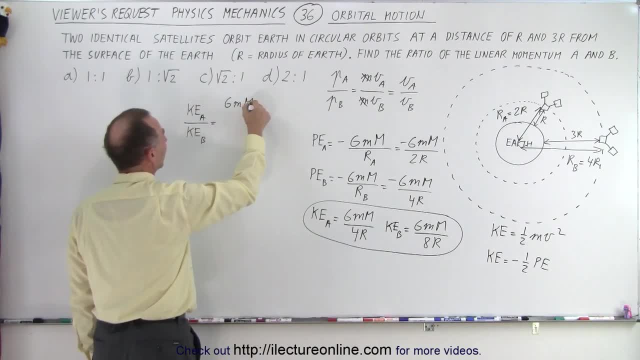 A would be G- little M, big M over 4R, divided by kinetic energy of B, which is GM, big M over 8R. So the GMM cancels out. We can divide both sides by R, So the R's cancel. 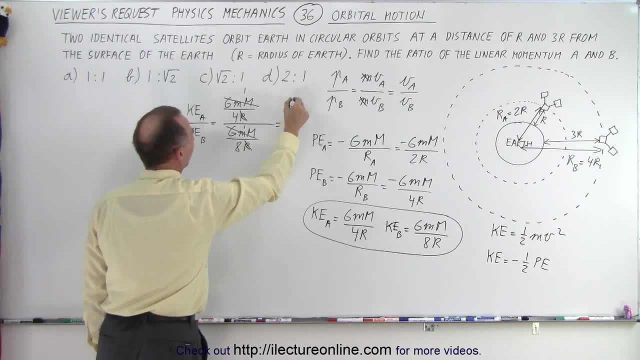 So all we have left is that the ratio is 1 over 4 divided by 1 over 8, which means it's 1 over 4 times the inverse of that, which is 8 over 1, which is equal to 2.. 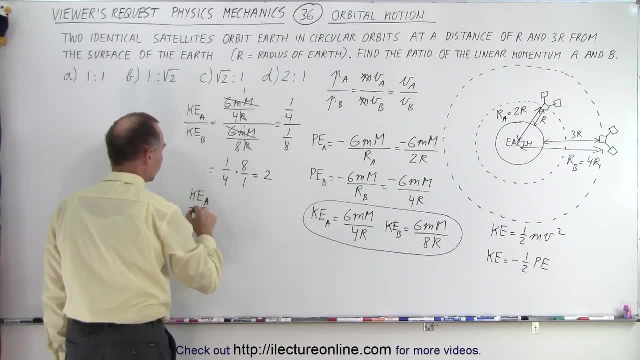 So the ratio of the kinetic energy of A to the kinetic energy of B is equal to 2 to 1.. So because we want to write it as a fraction, 2 to 1. Of course we're not looking for the kinetic energy. 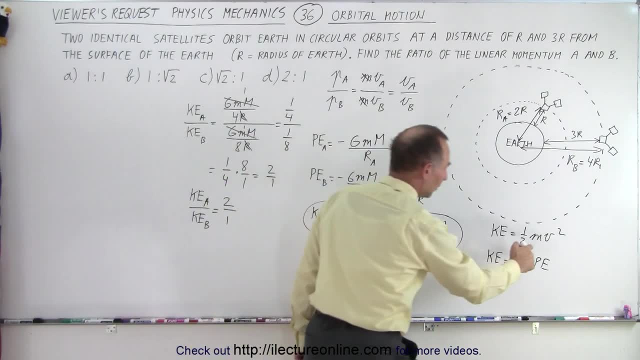 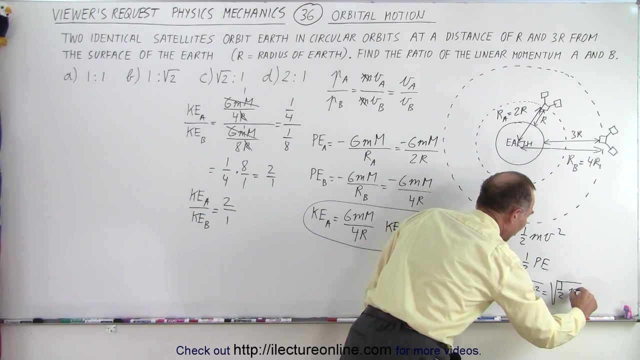 We're looking for the velocity. So then let's take this again and take the square root of both sides, which means that the square root of the kinetic energy is equal to the square root of 1 half M V squared, which is equal to the square root of 1 half M times V. 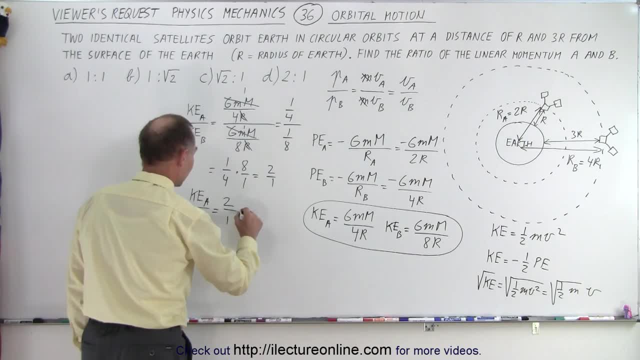 So now we can replace kinetic energy by that. So that means that this is equal to- Let's see here- The kinetic energy of A. Oh, I think what I should do. So, of course, take the square root of both sides first. 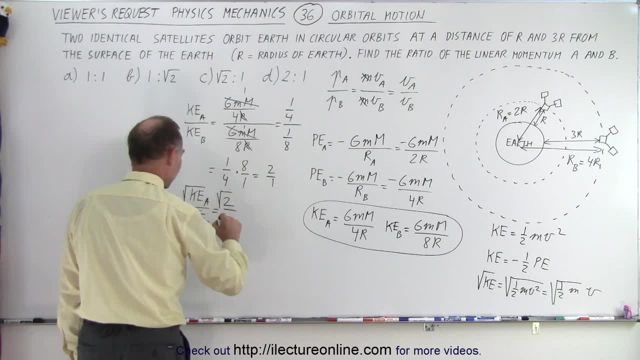 So take the square root of this, the square root of that, the square root of this and the square root of that. So now we know that the ratios of the square root of kinetic energy of A to the kinetic energy of B is the square root of 2 to 1.. 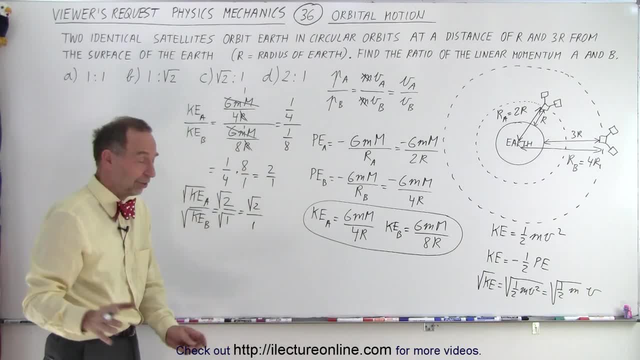 So it's equal to the square root of 2 to 1, because the square root of 1 is still 1.. Now we can replace that by that quantity. So now we have the square root of 1 half M times V A, divided by: 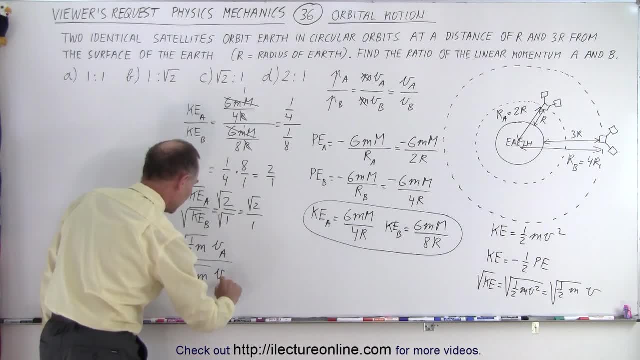 the square root of 1 half M times V B, because that's equal to the square root of kinetic energy of A and B, is equal to the square root of 2 over 1.. And then, since this cancels out, we now have the ratios of the velocity of A to the velocity of B. 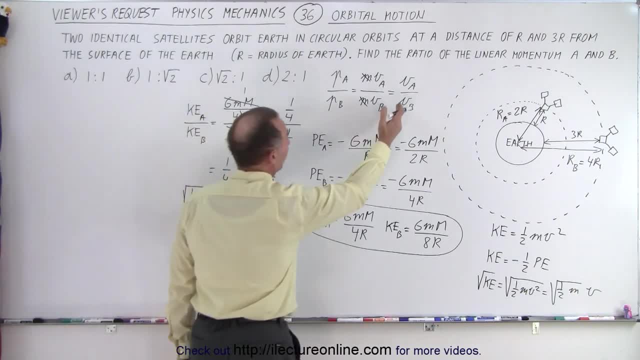 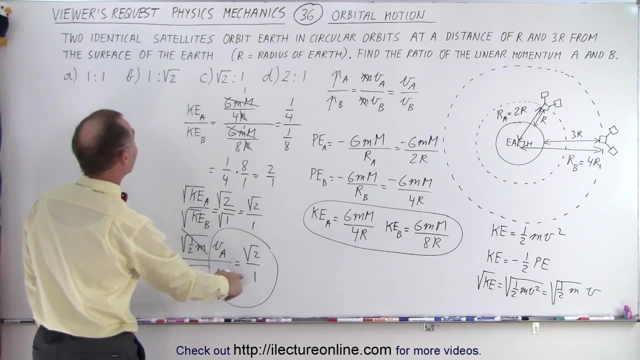 being equal to that ratio. right there, And remember that that is proportional to the ratios of the linear momentum. Now we look up here and is there an answer that looks just like that? And the answer is yes. right here. The answer C is indeed the square root of 2 to 1.. 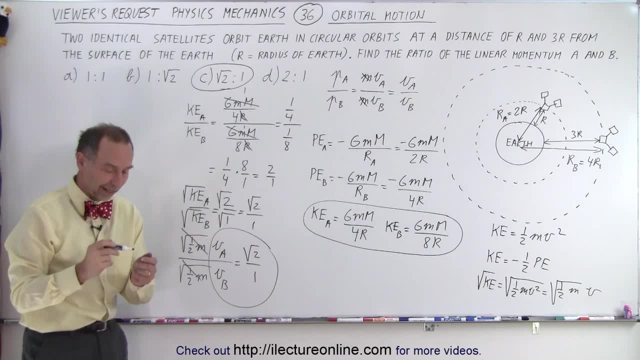 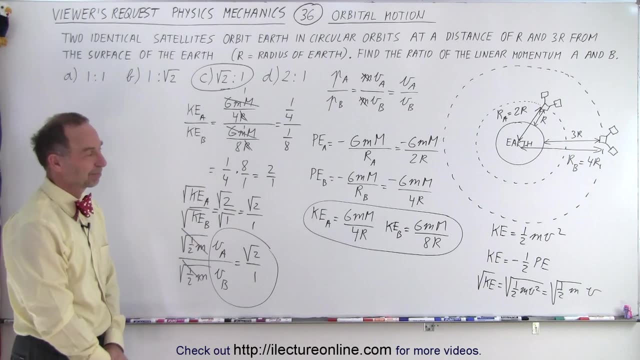 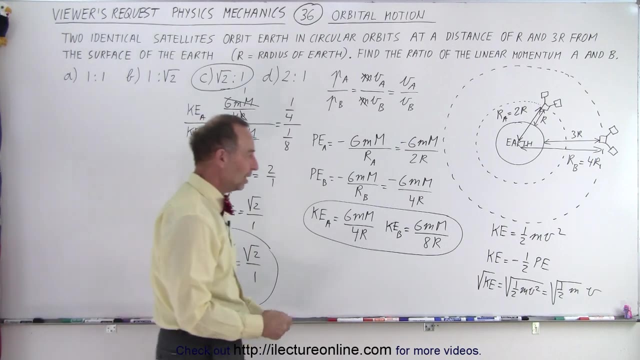 And that's the ratio we found between the two velocities of satellite A and B, And that is how it's done. How did we get that kinetic energy is equal to 1 half potential energy? Yes, how did we get the relationship between the kinetic energy and the potential energy? 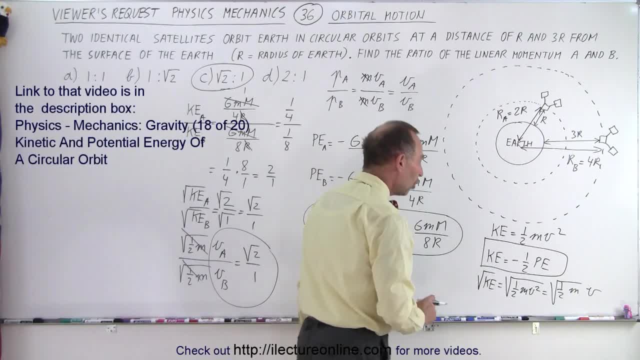 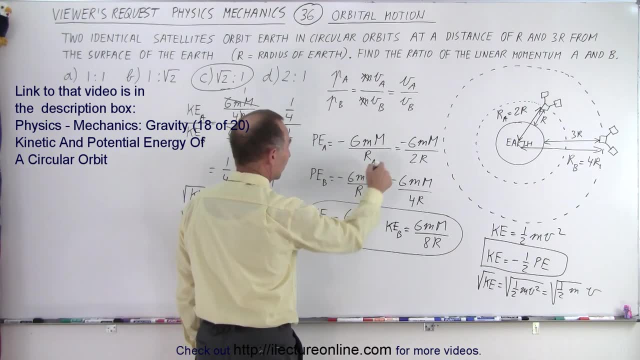 That's this thing right here. So it turns out- and we have that in some of our other videos- if we calculate the potential energy right here and then we calculate the kinetic energy of a satellite, which is equal to 1 half mv squared. 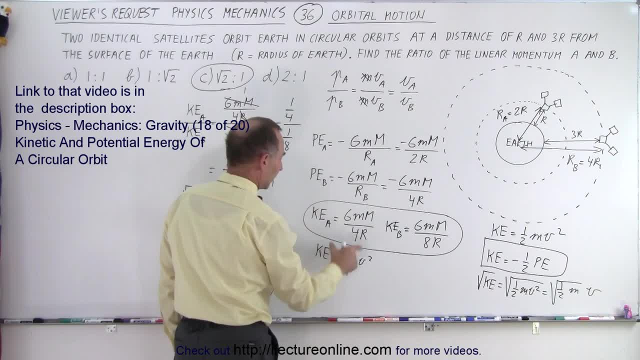 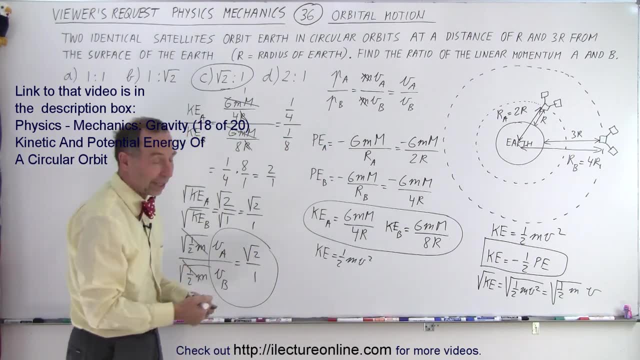 if we now compare this to this, if we compare these two to one another, we find out that the kinetic energy is equal to negative 1 half tons of potential energy. So I could show that, but that would take an entire video again to do that. 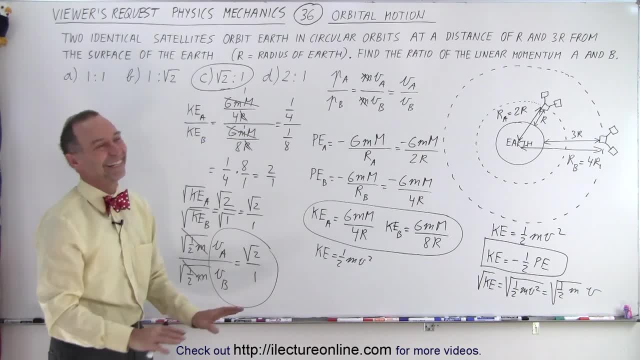 But yes, What's the algebra Plus a little algebra. Actually, you need to see it, but we do have that on video if you want. In our orbital motion and gravitation videos in physics we do have the explanation of how that's done. 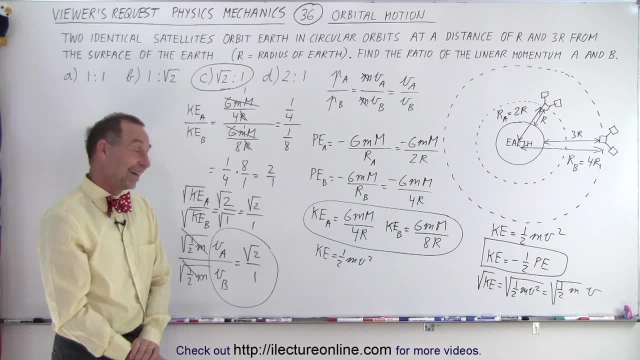 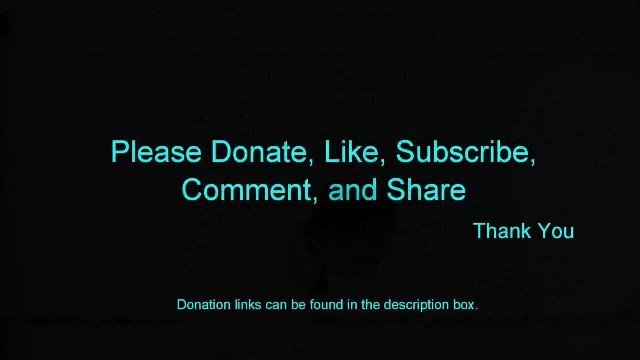 Okay. Okay, Because I didn't remember that. It's very handy if you remember that. If you don't remember that, then you have to calculate it right. But that's indeed the case In orbital circle, orbital motion. that is always the case. 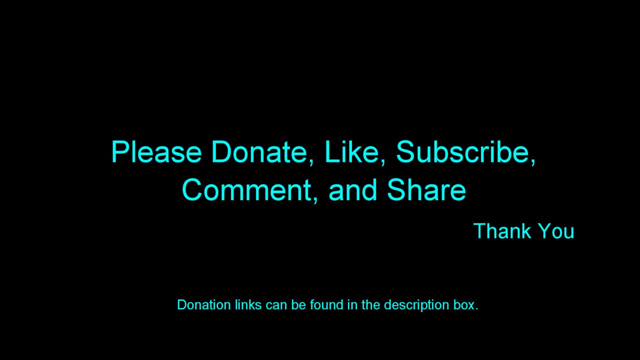 Okay, Okay, Okay. So we do an orbital motion and we calculate this, And now we're going to see how this works, And then we're going to see the difference between a horizontal pendulum and a vertical pendulum. Remember, you can't use a vertical pendulum. You're just going to use a vertical pendulum. You're going to do this. You're going to put the pendulum in the orbit of the Vertical pendulum. So that's what you're going to do. This is the vertical pendulum. Here's the vertical pendulum, And you're going to do it. 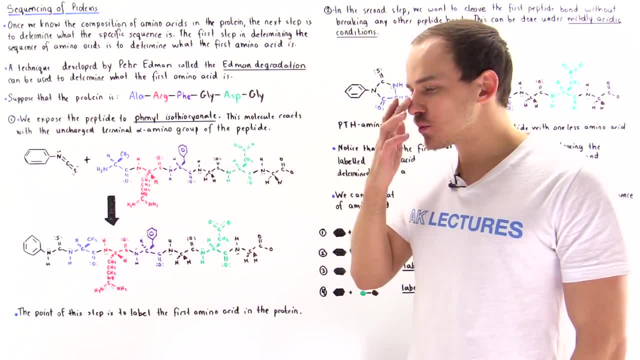 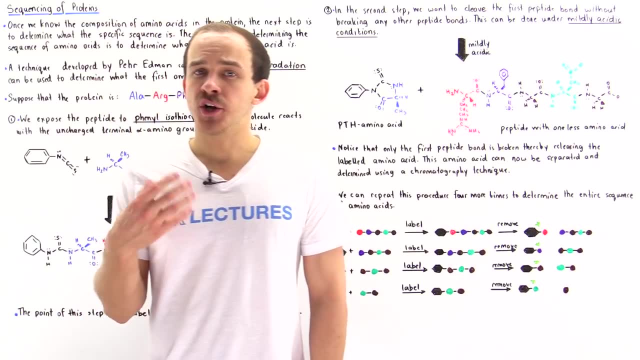 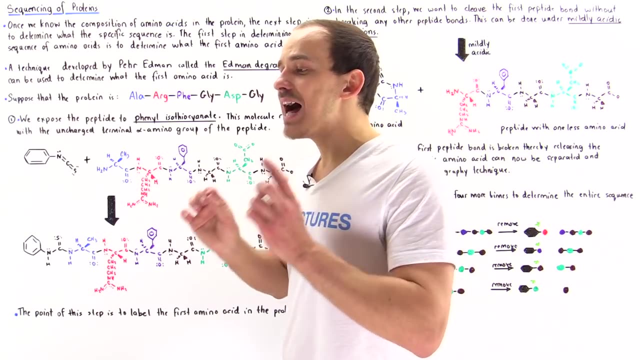 Previously we said that if we purify our protein that we want to study and we don't know anything about that protein, then the first step is to basically determine what the composition of amino acids is inside that protein, and that involves determining not only what types of amino.